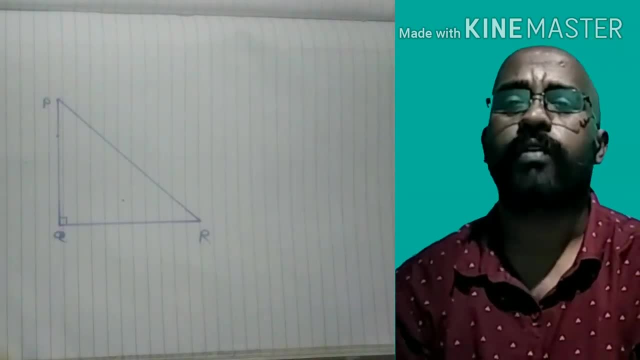 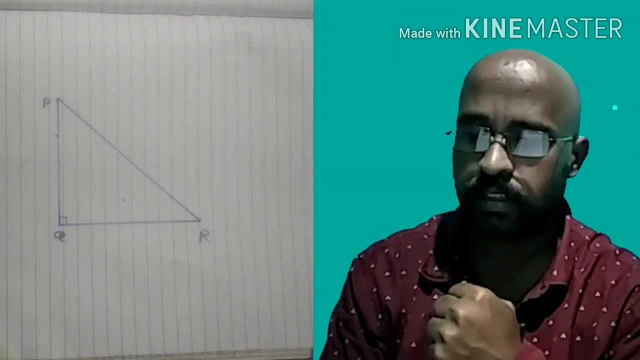 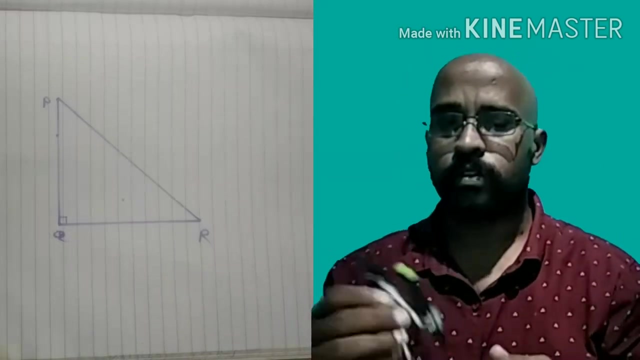 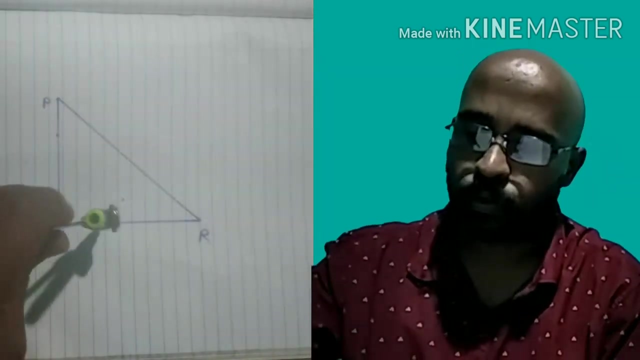 So PQR is a right angle triangle. Ready now What we have to do? Draw in circle. How do we locate in center? We have to draw angle bisectors. Can we bisect angle? Definitely, yes, Let's bisect. Let's first bisect this angle Q. Once again, same step. Take any random distance in compass. Okay, Draw two arcs on two arms of angle Q. Okay, 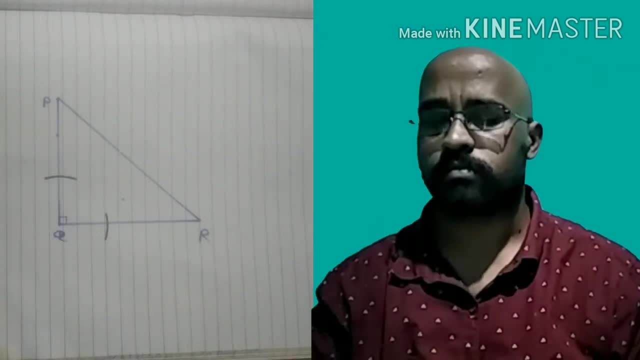 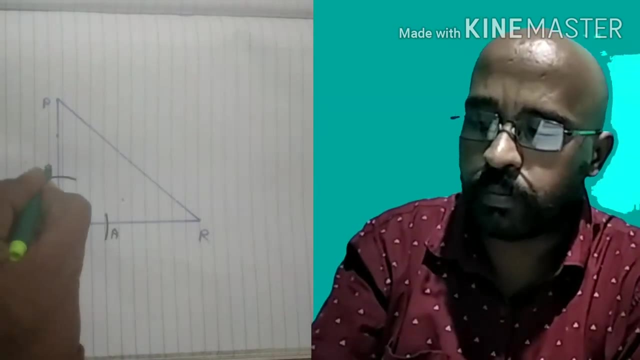 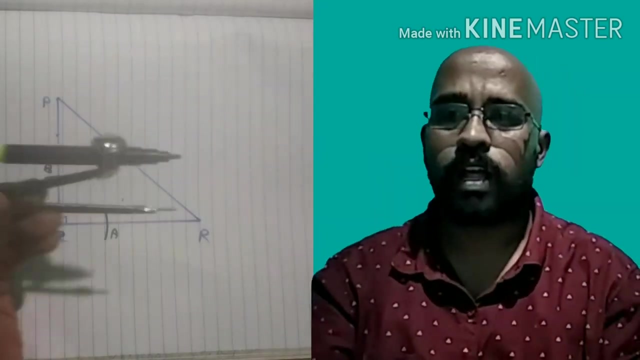 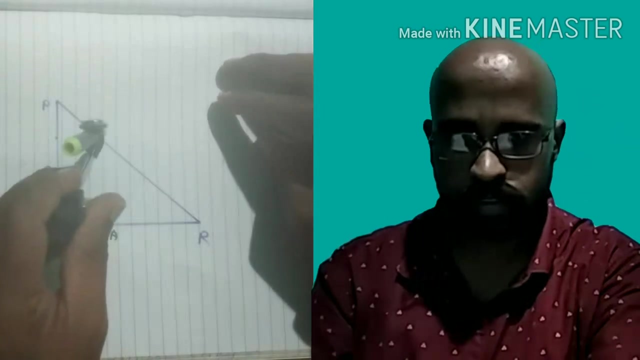 Give any appropriate names to this intersection point of arms, Arms and arcs. Suppose this is point A, This is point B. Now, from these two points we have to draw two arcs. So let's increase the distance such that the projected arc will go out of the triangle. Okay, Students, I have increased this much distance. 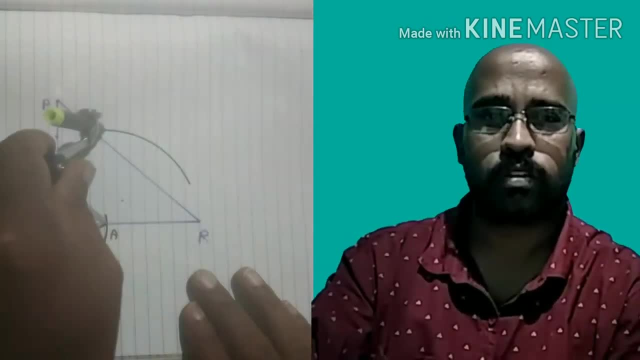 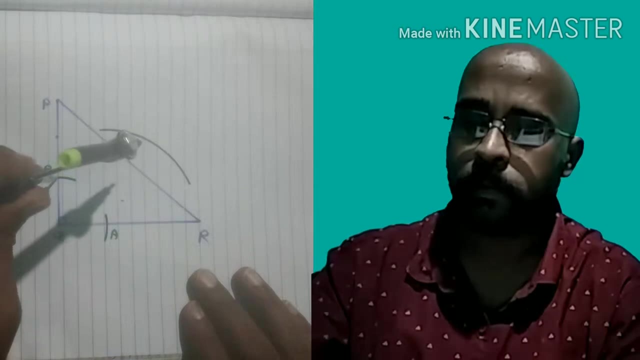 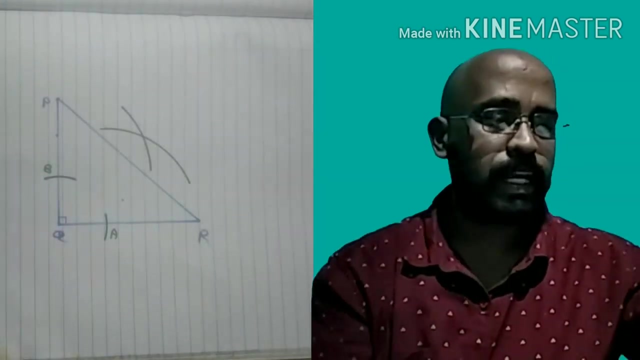 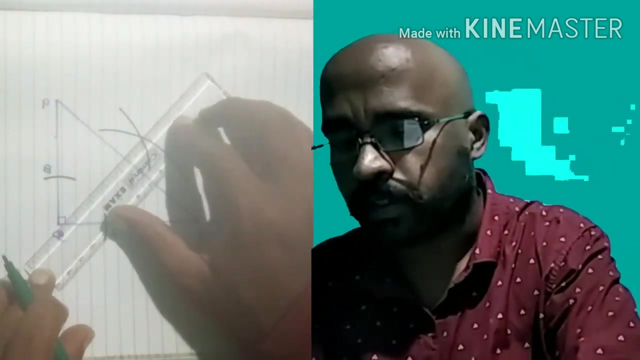 Now, from point A, I will draw one arc. I have drawn it Now without changing this distance. without changing this distance, I will draw the arc from point B. Got it Now. locate this intersection point of two arcs. Join that intersection point with point Q. We are just following same steps repeatedly. 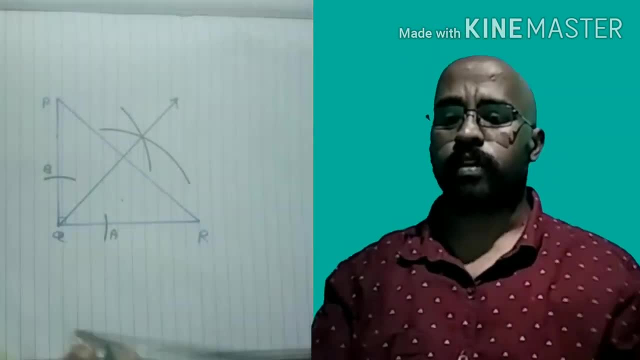 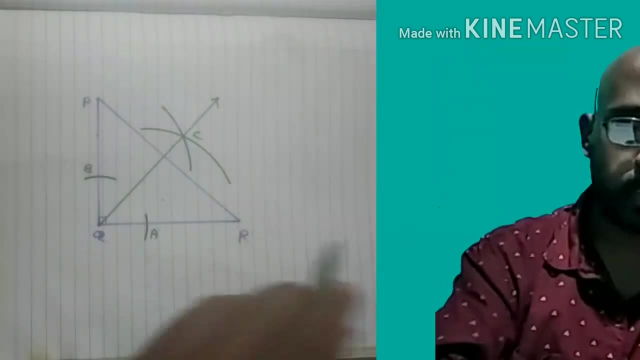 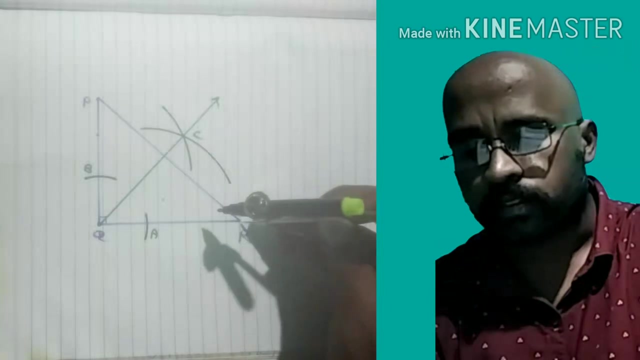 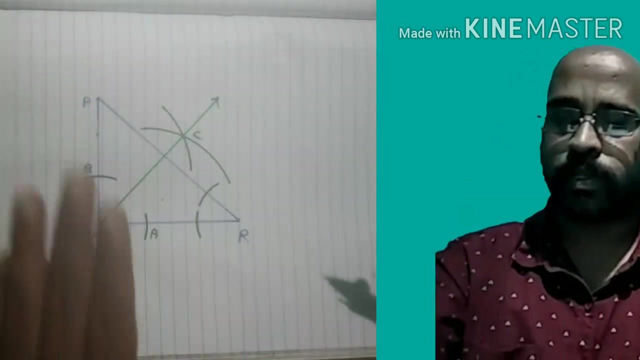 Okay, So this suppose C, QC is angle bisector of angle PQR. Similarly, let's draw angle bisector of angle R. First step: take any random distance taken from point R, Draw two arcs on the two arms of angle R. We bisected this angle, Yes, So this and this two arms needs to be bisected. 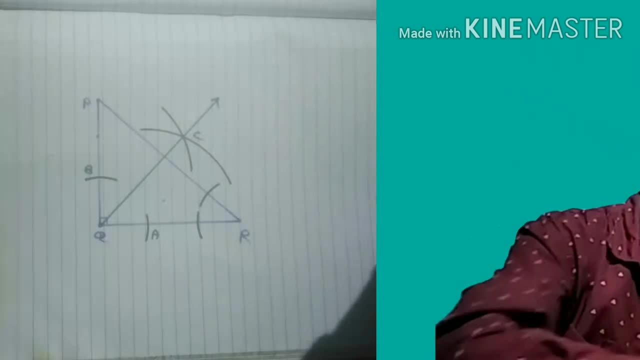 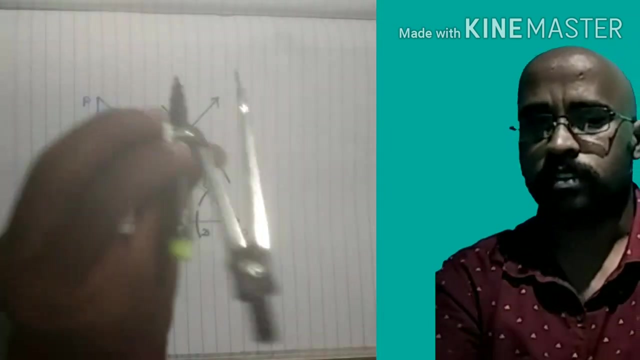 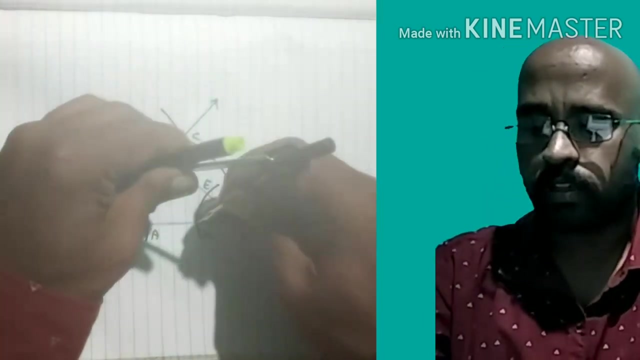 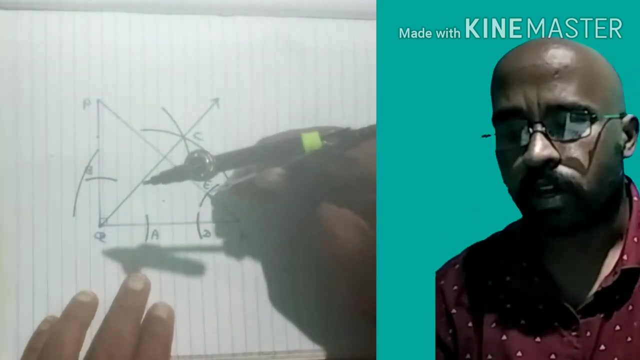 Intersected by this arc. Now give them names. Suppose this is point ABCDE. Now increase this distance such that it should go out of the projected arc, will go out of the triangle, So I'll increase it little bit and draw one arc. Okay, guys, Now from point E, draw another arc intersecting previous arc. Got it? 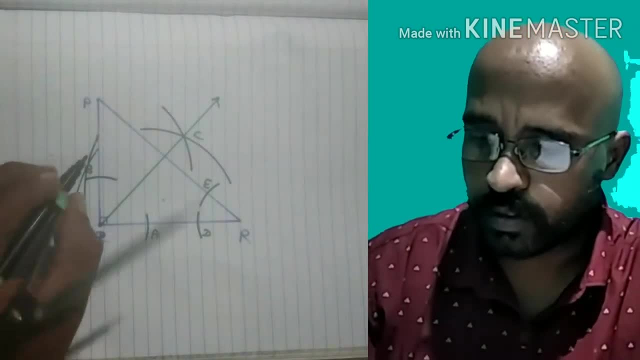 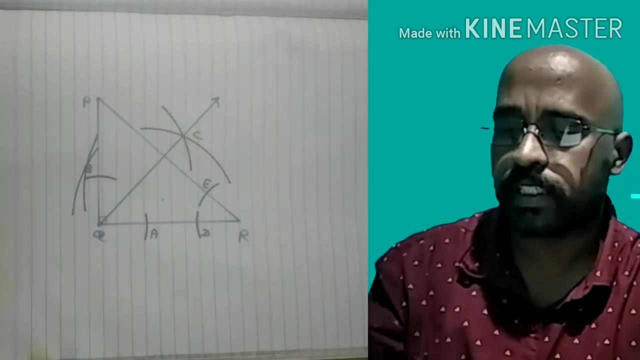 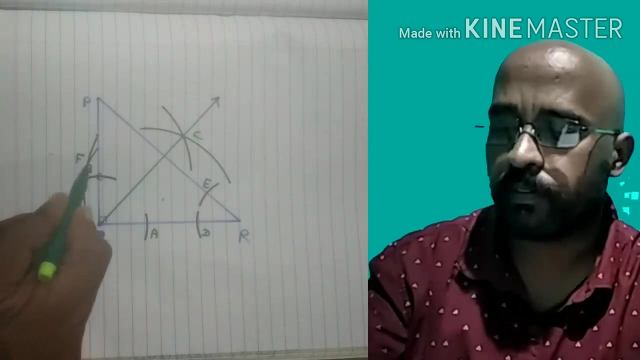 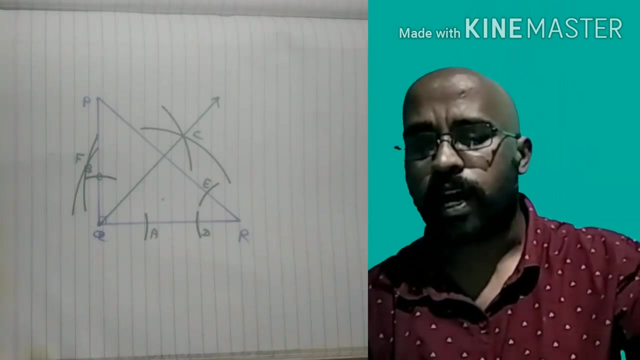 So this point, This point, is the intersection point of these two arcs. Let us give it a name: ABCDEF. Students don't get confused between this point B and F. B is this point and F is this point. Okay, So let's draw one array connecting point R and F, which will be the angle bisector. 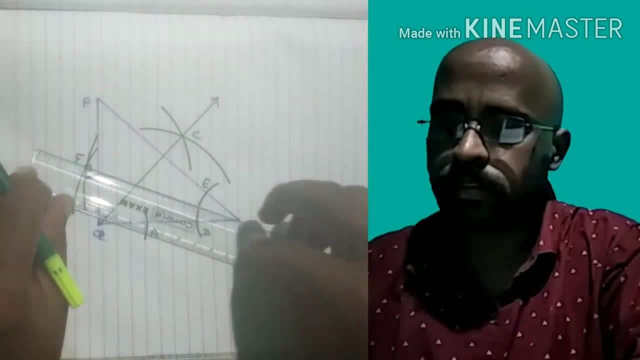 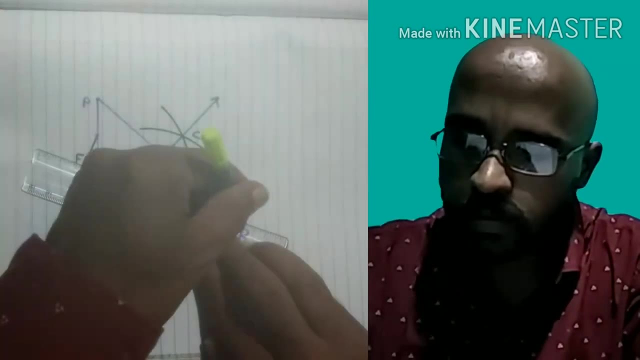 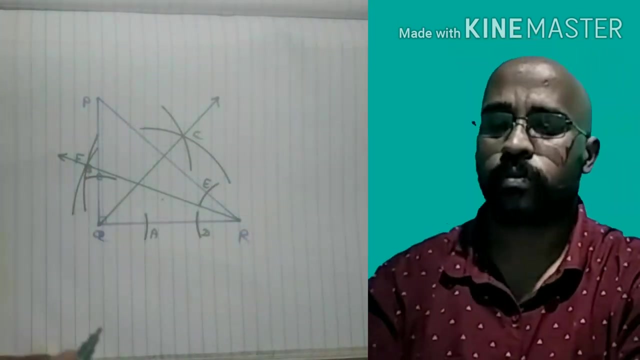 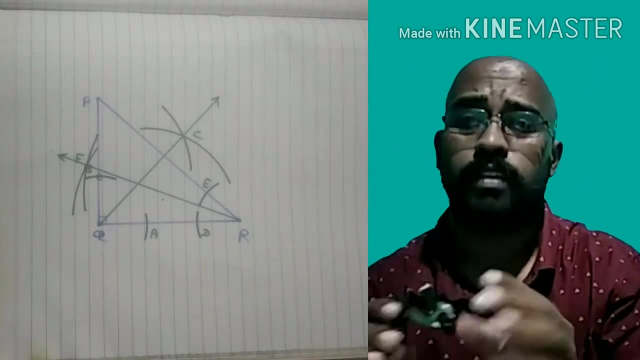 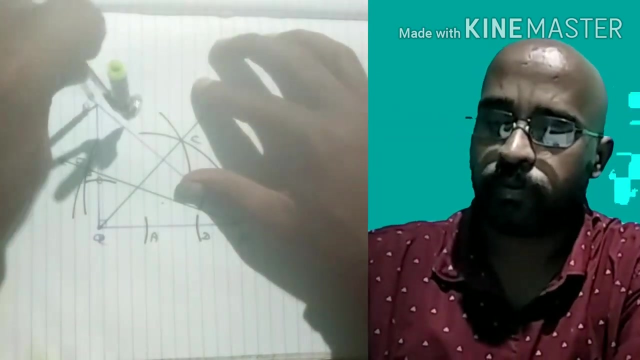 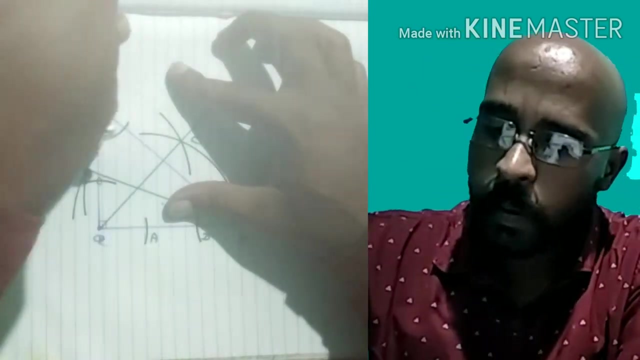 etc. Done Okay, And final step is we have to bisect this angle, QPR. Just same step we have to follow repeatedly. One of the is just a lesson: no calculation, nothing, Very few steps, Few drawings. drawing steps have to follow repeatedly. So I draw one arc intersecting these two arms. 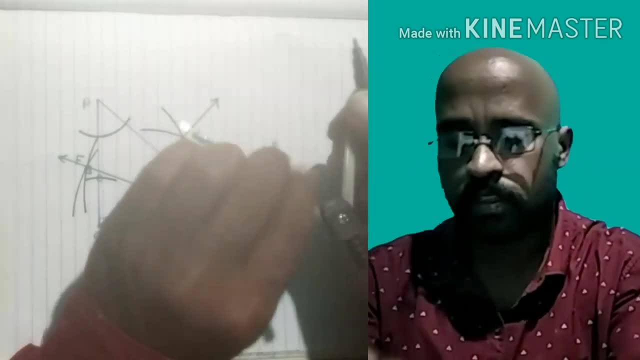 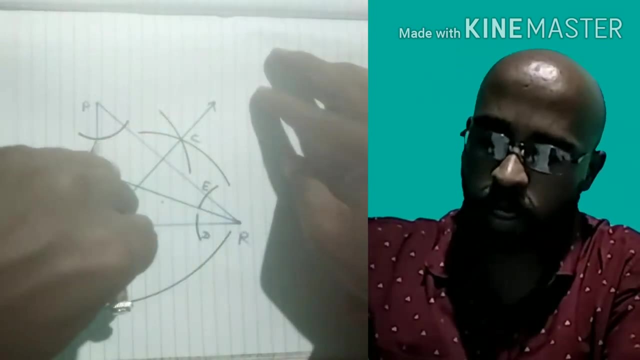 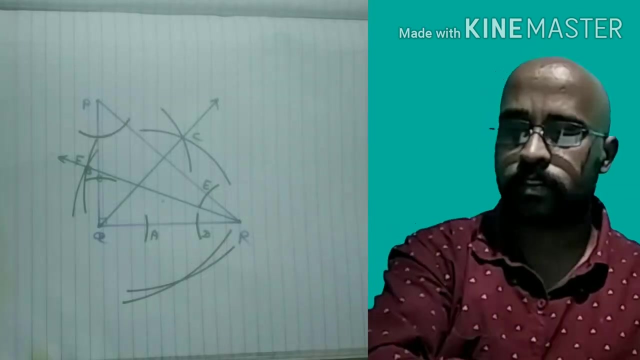 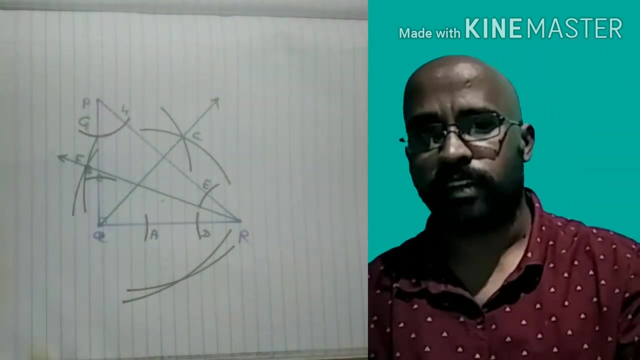 of angle P, then increase the distance and draw two arcs out of the triangle. Okay, students, suppose these two points were point G and H. you can give any names, but ABCD is easy. right, And connect this point Automatically. 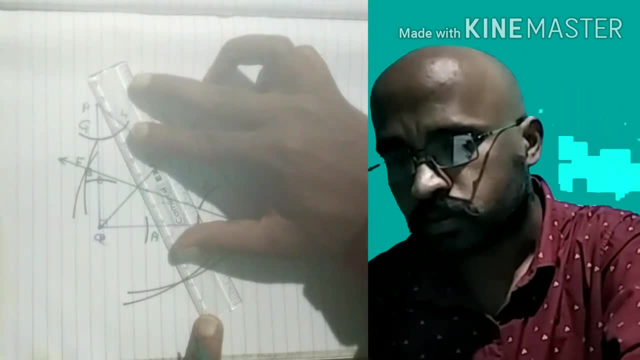 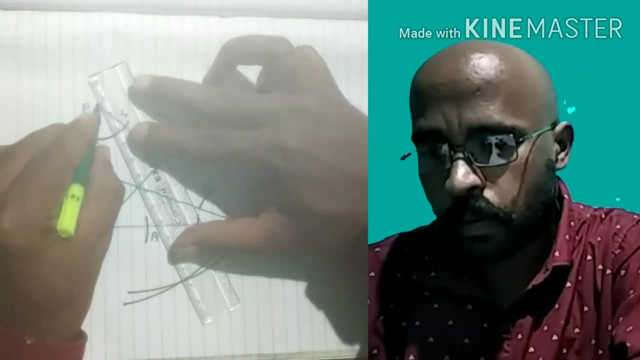 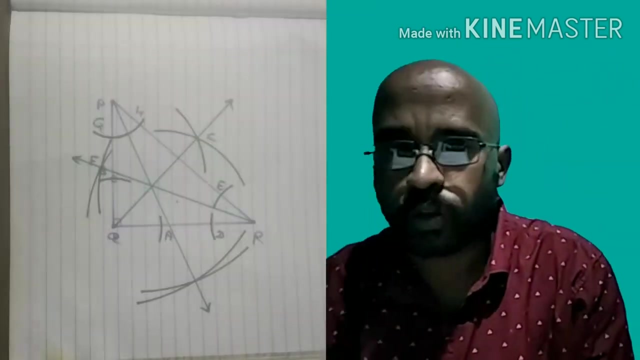 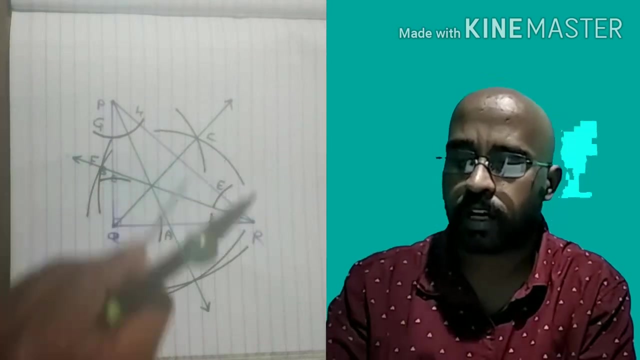 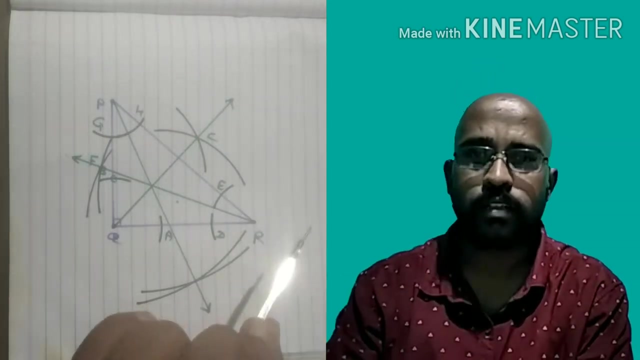 this point will go through the interior of the triangle. Okay, so why I told you to increase the distance in the compass so that this projected arc will go out of the triangle? Because, students, either it is acute angle triangle, right angle triangle or obtuse angle triangle, There in center always will. 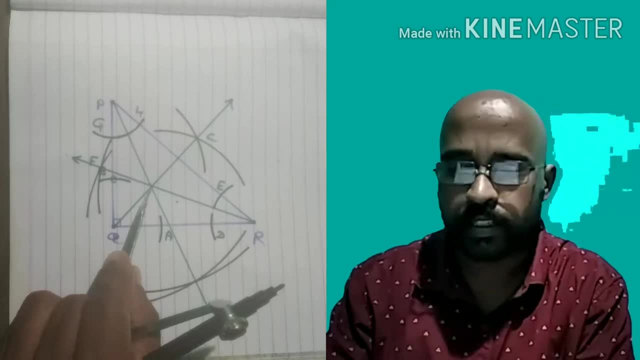 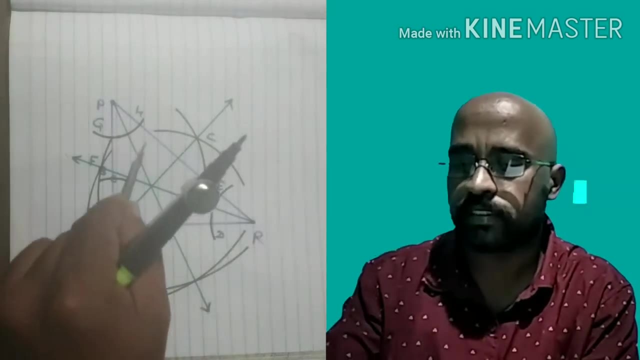 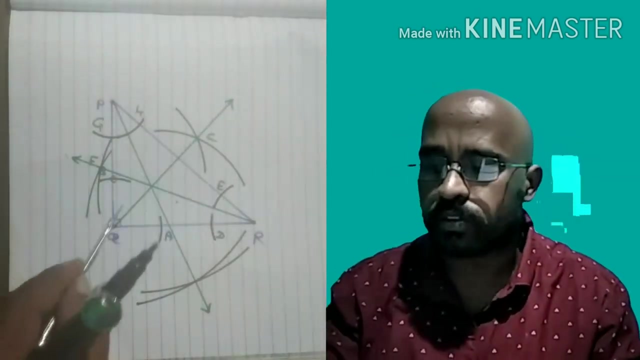 be in the interior of the triangle, So in center will be in the interior. if this intersection point of arcs also will be in the interior, then here will be lot of arcs in this interior. here will be lot of arcs, Suppose these two arcs shifted here. here will be two arcs, Suppose 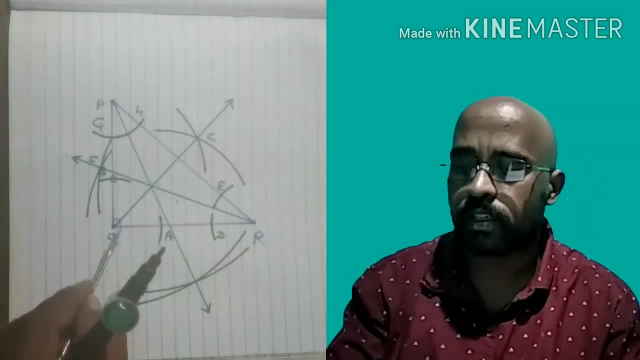 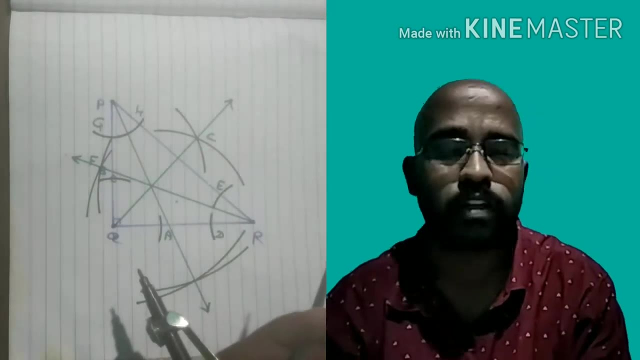 these two arcs shifted in the interior, here will be two arcs. these two arcs shifted here, here will be two arcs. So there will be lot of arcs and after that we have to draw circle also. So it will create confusion. So to avoid that confusion, take distance such that 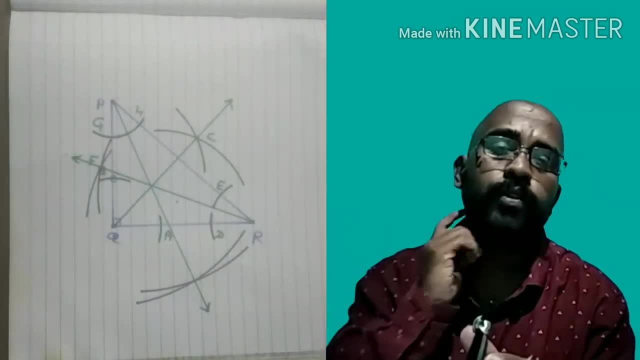 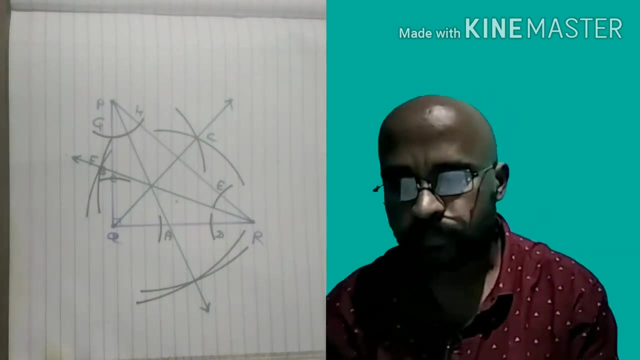 projected arcs will go out of the triangle. You may observe, you may cross check this with previous video also there we draw acute angle triangle and its in center and in circle. there also in center and in circle. there also in center and in circle. there also in center and in. 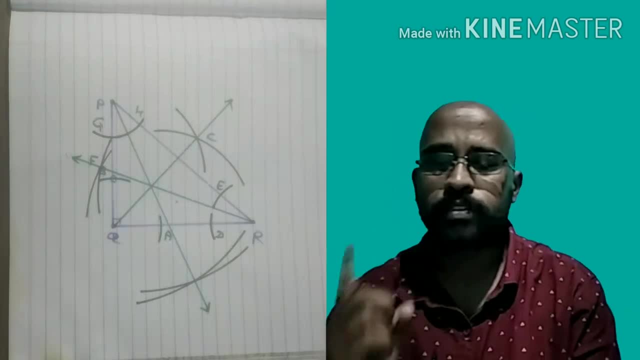 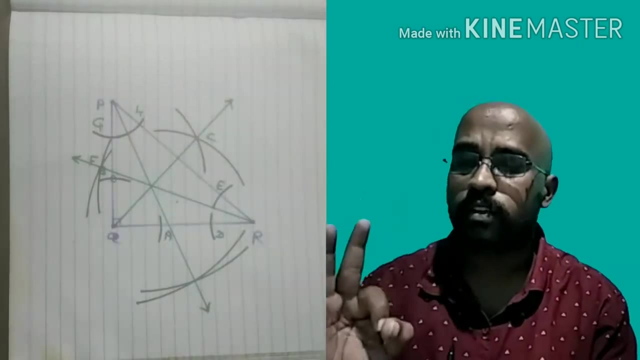 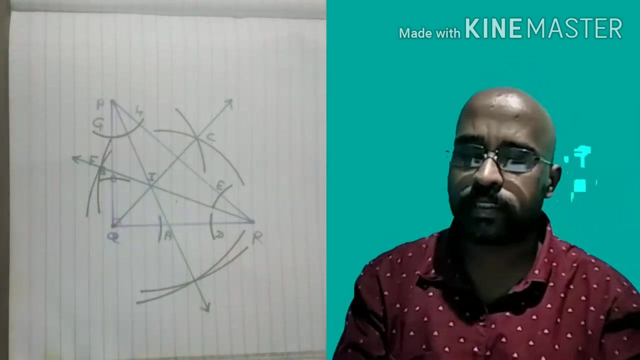 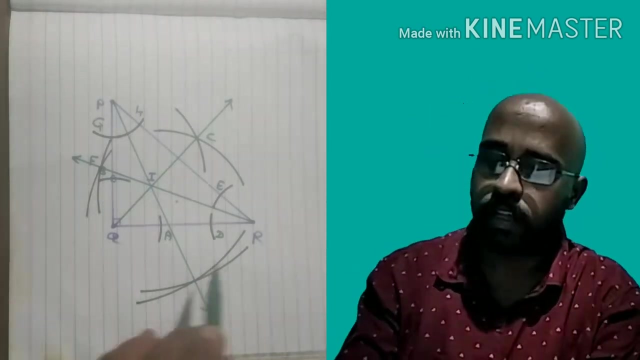 center was in the interior, so let's continue. first step is draw triangle that we have drawn. second step: bisect all the angles that we have done. third step: from this in center- let's name it as i so- from this in center, we have to draw one perpendicular, either on any one side, either 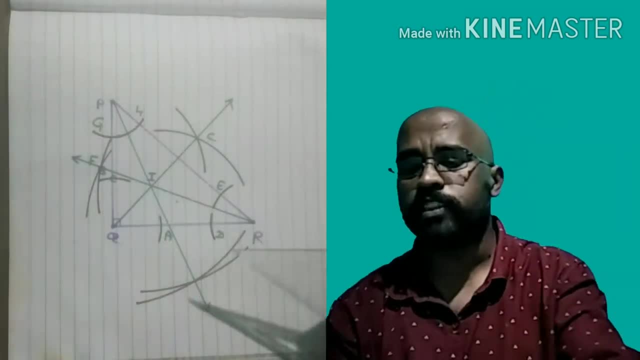 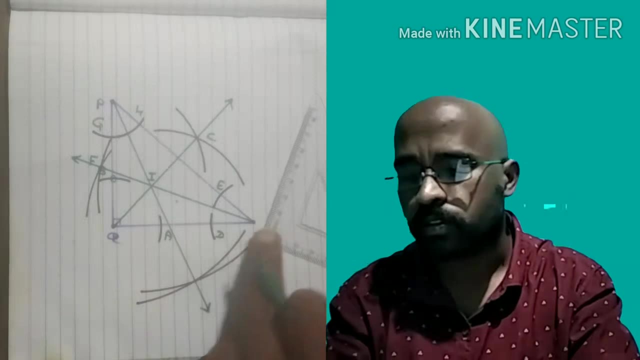 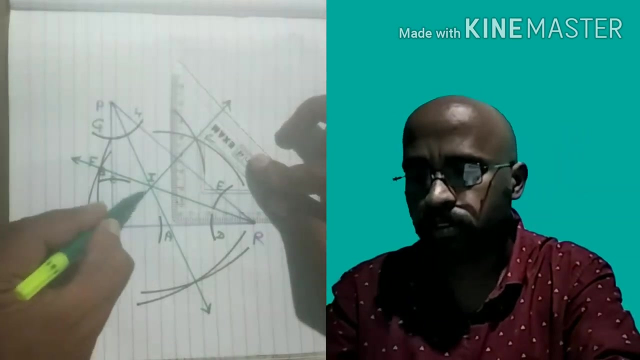 on side qr, pqr, pr. but it's easy for us to draw qr, so let's draw a perpendicular on qr by using set square. what we have to do: align this base on the side qr properly. i have aligned here, first thing. second thing: its height should touch to this point r, so slide it such that. 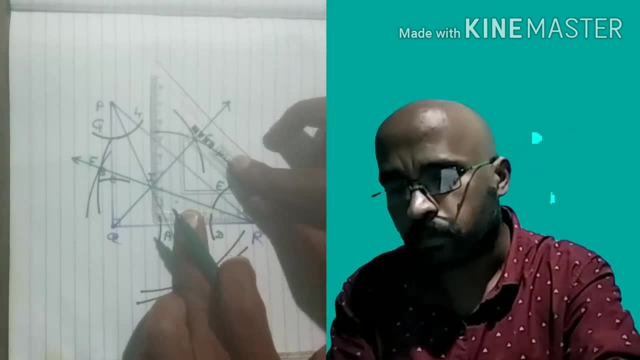 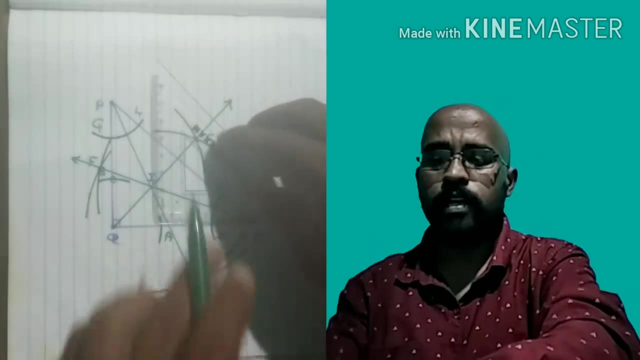 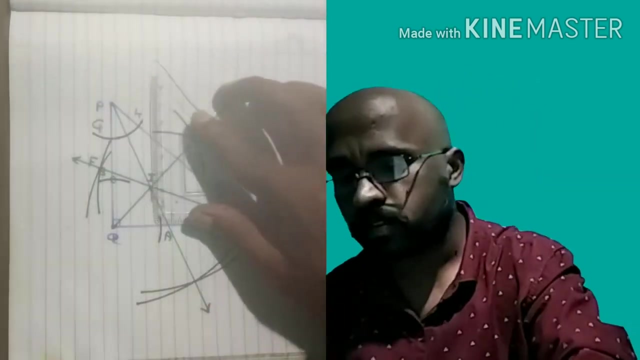 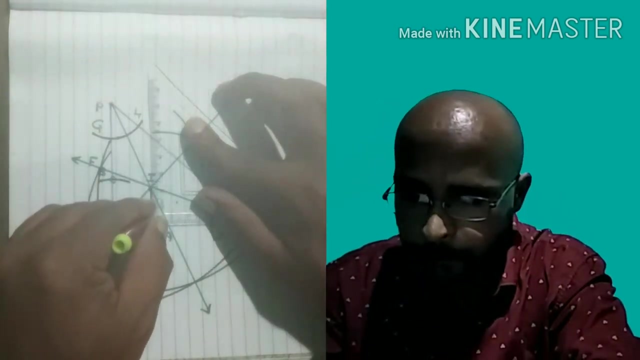 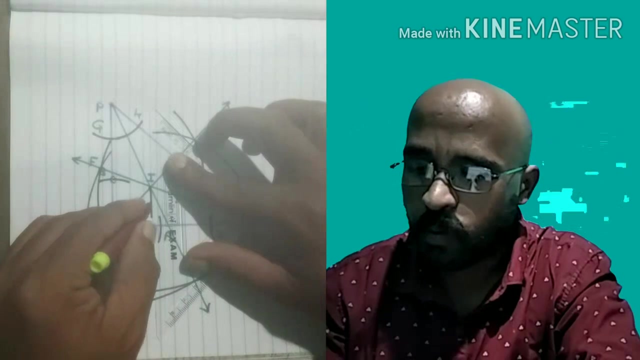 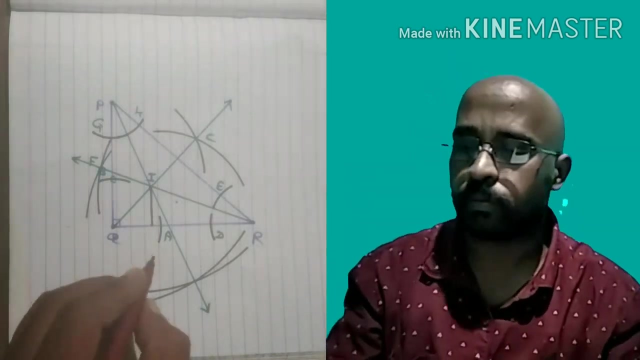 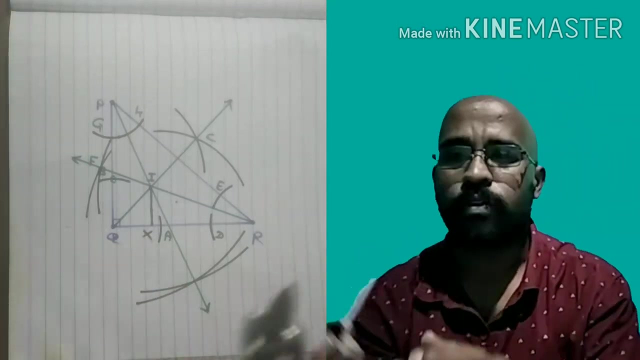 base is aligned to side qr and height is touching to the side point i. now, from this point, we have to draw one perpendicular. so let's draw a perpendicular. okay, now we have to take distance in the compass. sorry, suppose this is point i x, this is point i x. we have to take the distance in the compass. 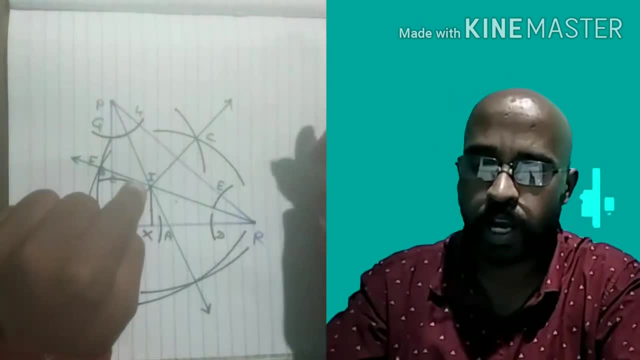 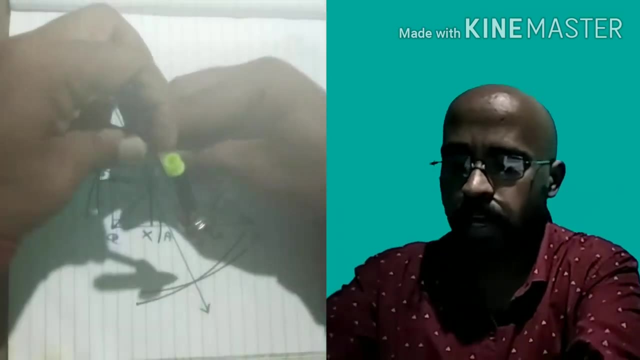 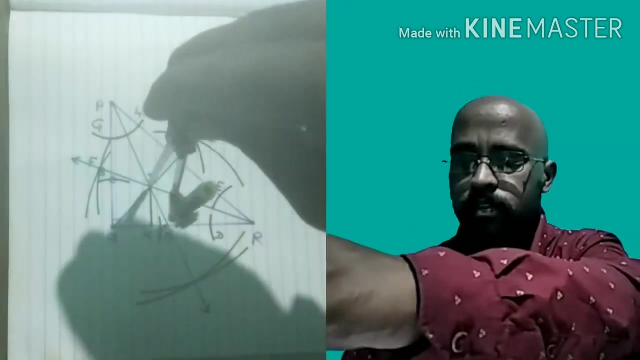 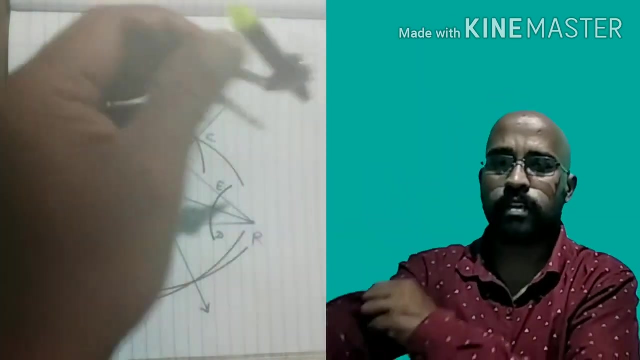 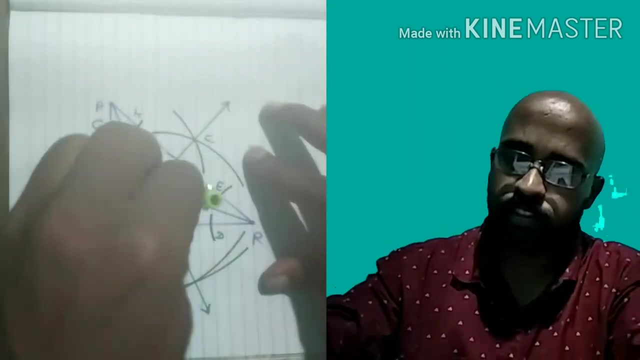 which is equals to point i. x means put this tip of the compass on i pencil tip of the pencil on x. so let's do it. i x, c. i have kept the tip of the compass on i and pencil on x. So Ix is the radius. Put the center, consider the center as I and draw a circle. So let's draw it.